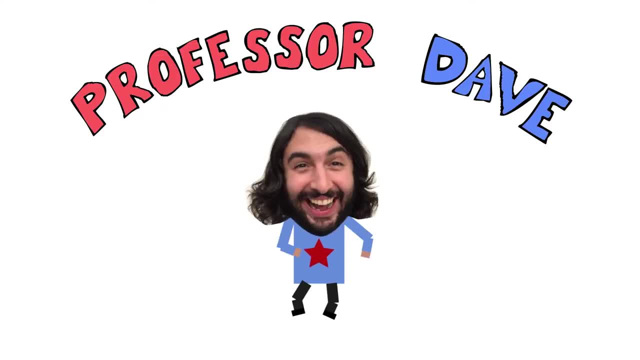 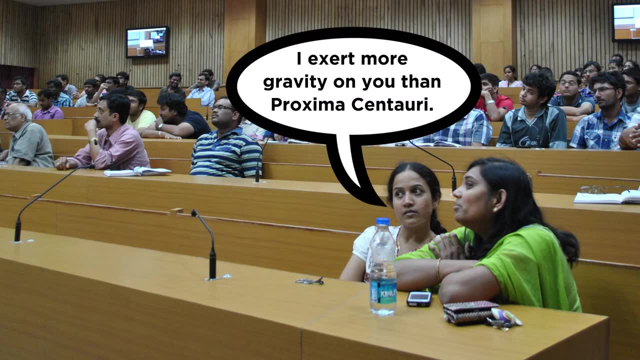 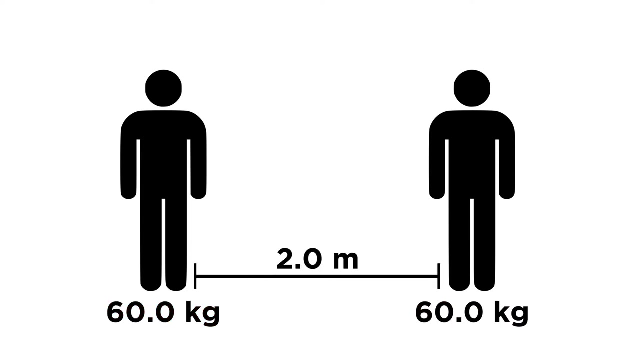 One day, in physics class, you're learning about gravity and your friend tells you that they exert a stronger gravitational force on you than the nearest star beyond our sun, Proxima Centauri. You have a mass of sixty kilograms, as does your friend who is sitting two meters away. 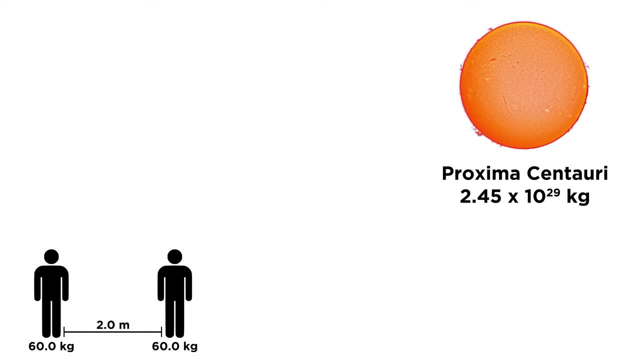 Proxima Centauri has a mass of two point four, five times ten to the twenty-nine kilograms, and it is four point zero one times ten to the sixteen meters away. So is your friend correct? Which exerts more gravity on you, your friend or the star? 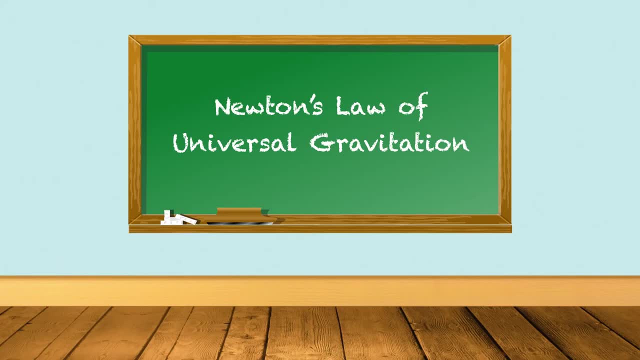 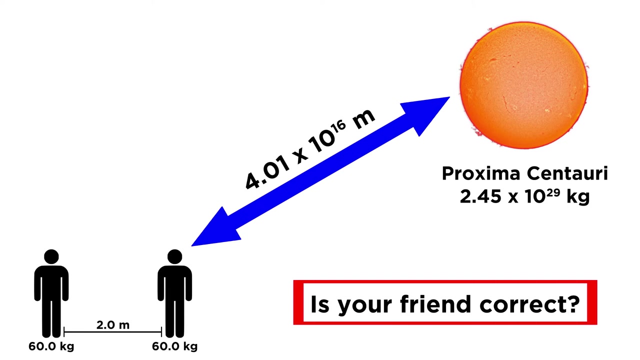 To answer this, we will need to use Newton's law of universal gravitation. so if you missed that tutorial, check it out right now. If you know what to do, give this calculation a try. This is easy to solve if we know this equation. 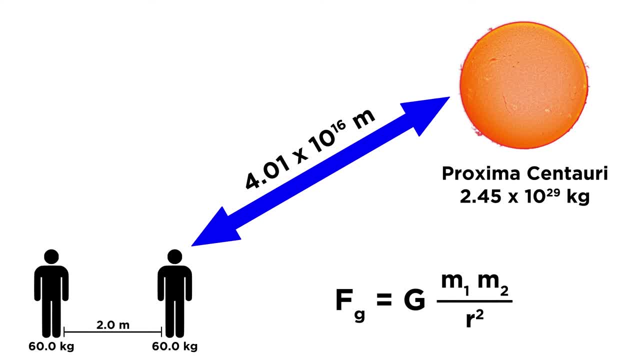 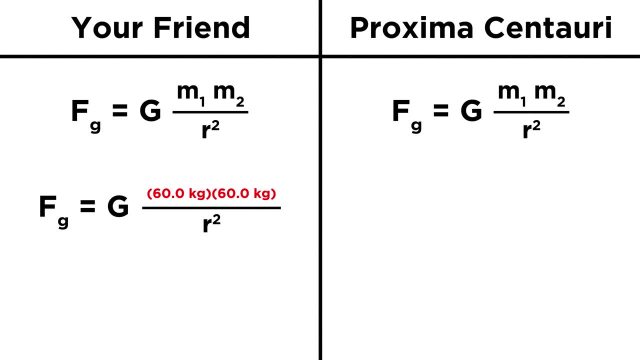 All we do is plug in the masses and distances involved, as well as the gravitational constant. First, for your friend, we plug in sixty and sixty as the masses and two meters as the distance between you. We square that and evaluate, and we should get six times ten to the negative eight newtons. 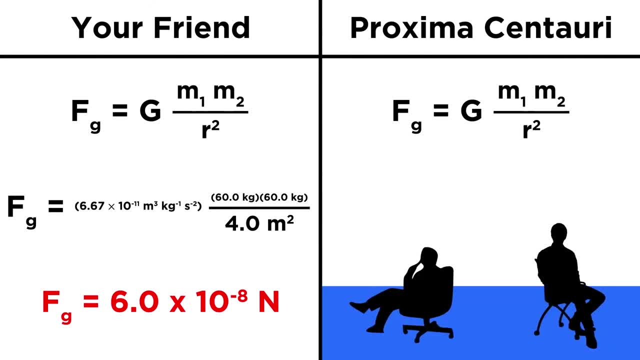 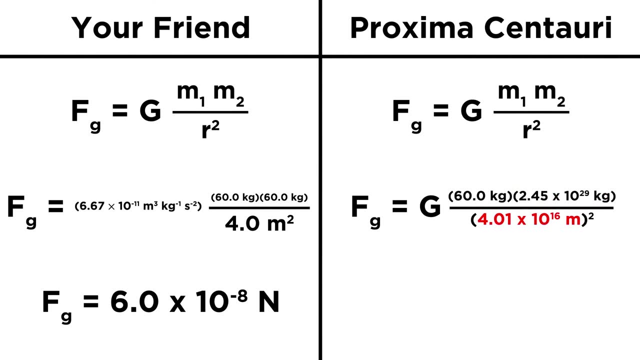 This is an extremely tiny force, which explains why people don't slowly drift towards each other when sitting in a room. Now let's do one for the star. We replace the mass of your friend with the mass of the star, But we also change this value to the distance to the star, so we have a huge number on top. 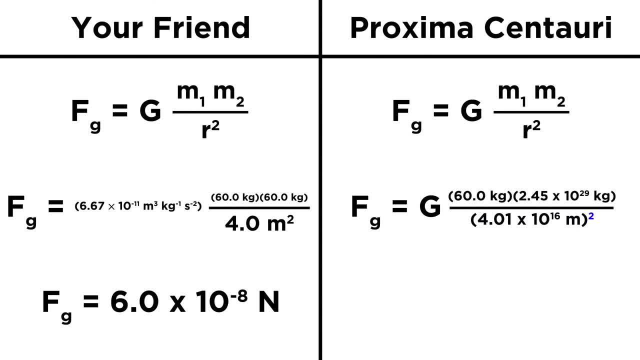 but we have a pretty big number on the bottom too, and we have to square it. So when we evaluate this, we get six point one times ten to the negative thirteen newtons. As small as the first number was, this one is a hundred thousand times smaller.